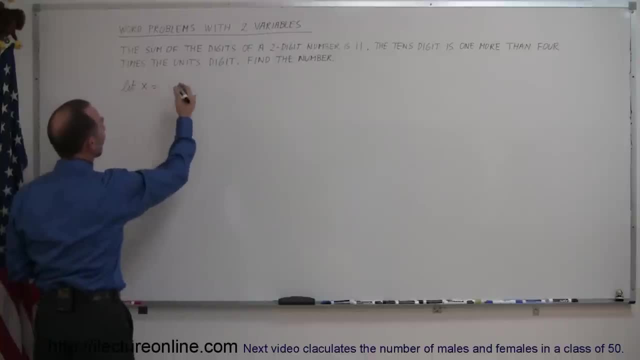 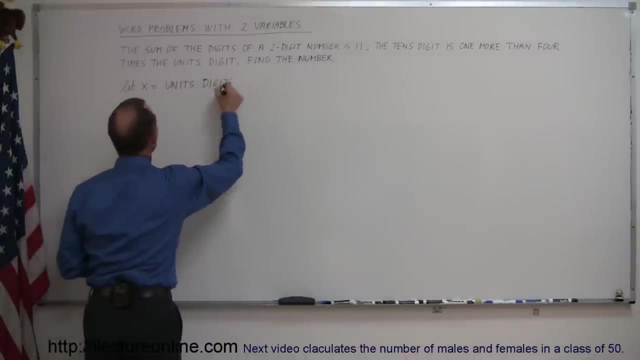 define them. You're going to say: let x equal and let's call x the units digit, and then we're going to use y and call that the 10. digit, so that the number that we have will kind of look like y, x. y is the tens digit, x is the units digit. and then they tell us the following: it says that the 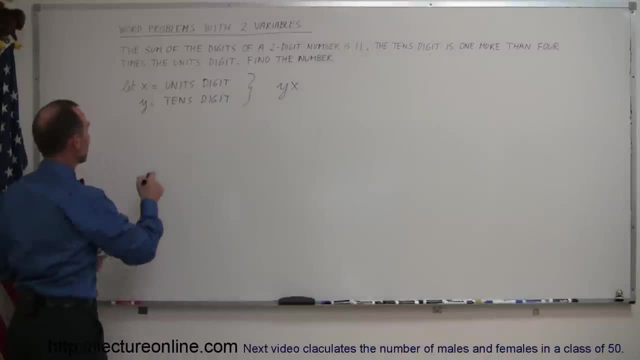 sum of the digits of the two-digit number is 11, which means that x plus y equals 11. and then they tell us that the tens digit is one more than four times the units digit. so the tens digit right here is y. so y is equal to one more plus one. then four times the units digit, four times x is the. 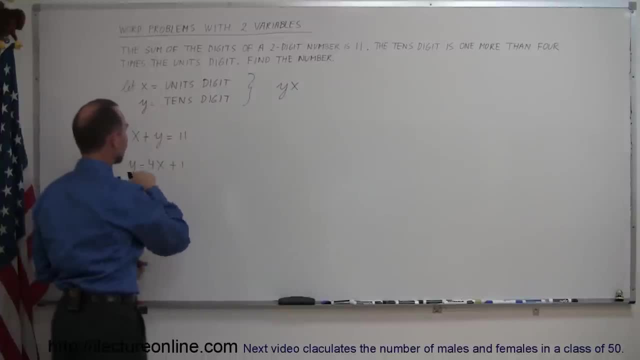 units digit plus one, that's one more than four times the units digit, and that's how you end up with your two equations. so now you need to solve these two equations simultaneously. there's different methods, but the one method here would, uh would be probably the the best one to use, which is: 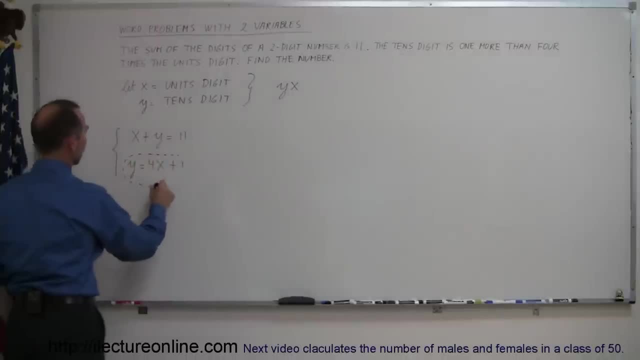 finding one of the two variables in terms of the other, and that's already in this form. y is in terms of the other variable- and then substitute that into your other equation. when you do that, you get the following: you get x plus y, being 4x plus 1 is equal to 11.. Notice that y is now replaced by the. 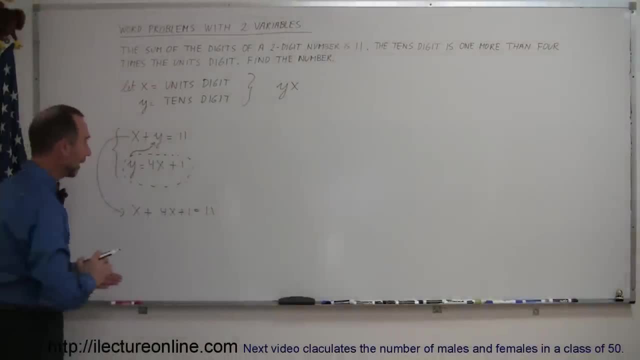 4x plus 1, and now you simply solve this equation for x. so this is equal to 5x plus 1, equals 11, combining the x's, bringing the y's and the x's together, and you get x plus y being 4x plus 1.. 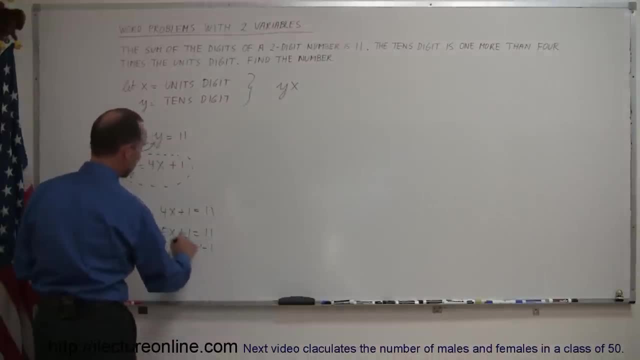 Bring the 1 across. this is 5x equals 11 minus 1. remember, when we cross equal sign, you change the sign and so we have 5x equals 10, dividing both sides of the equation by 5, the coefficient front of x, and that means that x equals 2.. Then we go back to what x represented. it represented the. 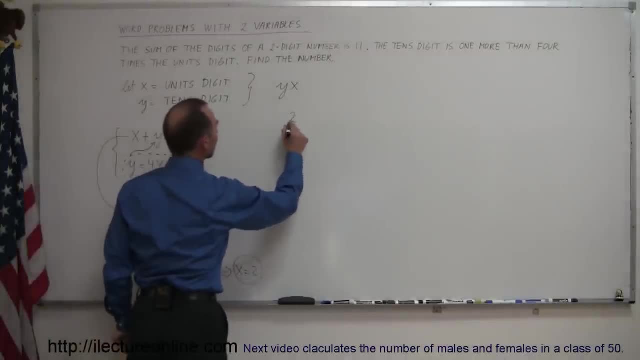 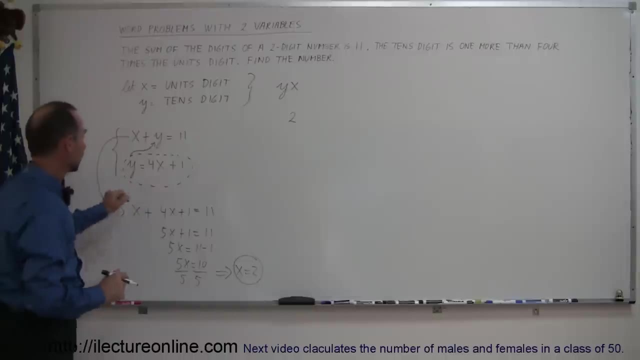 units digit. so the number then becomes 2 in the units digit. we still have to figure out what the y is equal to. Well, we can go back to one of our equations, and we can go back to one of our equations right here, this one right here, and we can say that y is equal to 4 times the units digit, which.